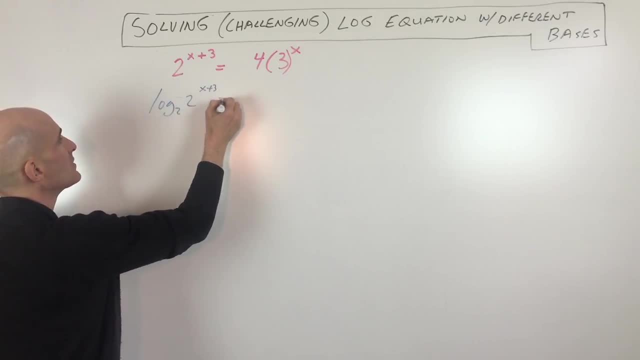 base 2 of 2 to the x plus 3 equals log base 2 of 4 times 3 to the x. Okay, so you're with me. so far we did it to both sides. we're keeping the equation balanced. But the log base 2 and the exponential 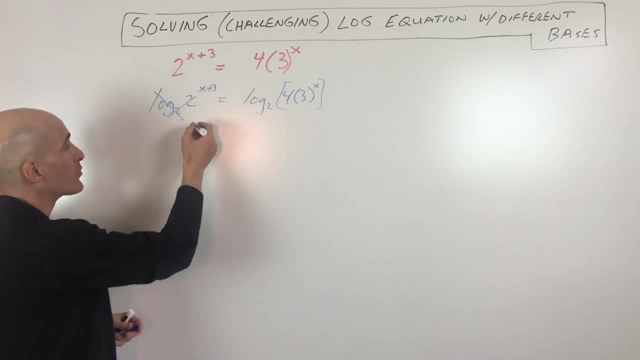 function base 2. those are inverses, so they cancel one another out and we're just left with x plus 3.. So we've eliminated one log, okay, and we've eliminated one exponential equation- okay, but we still have this group here to work with. So 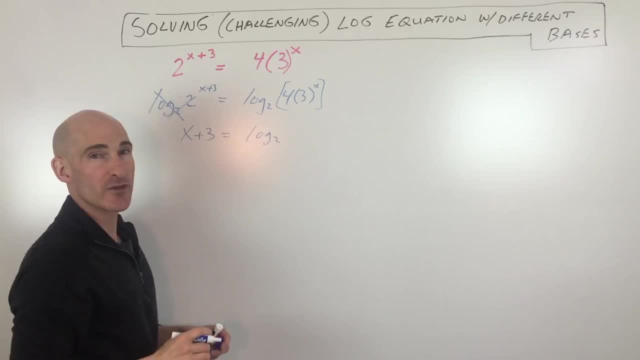 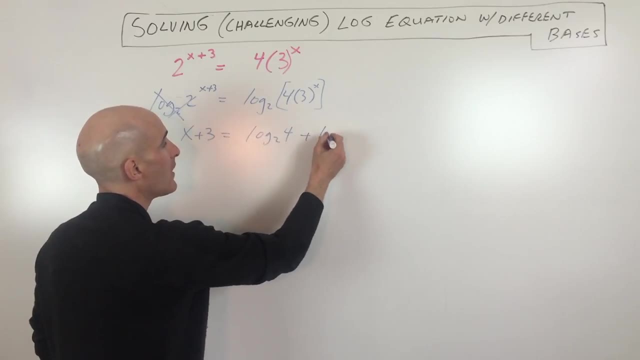 what we're going to do now is because these are multiplied together, the 4 and the 3 to the x. we're going to use the properties of logs to expand this. So this is going to be log base 2 of 4 plus log base 2 of 3 to the x power. Okay, now we're going to continue on. we're going to take 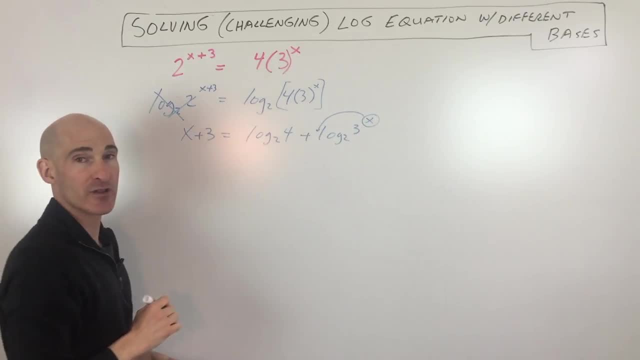 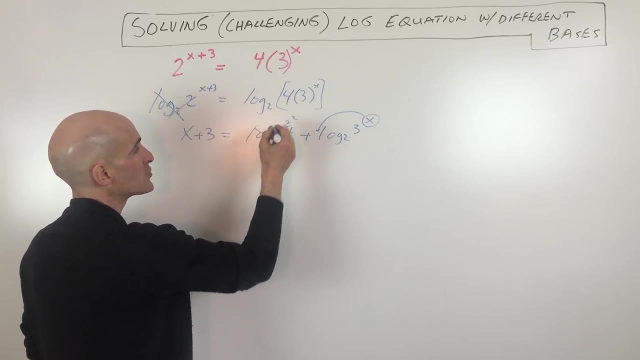 this exponent: use the power rule for logs. you're going to bring that down in front of the log. okay, 4 is really like 2 squared. okay, so log base 2 and exponential base 2- those cancel, Those are inverses. so we're left with 2.. Over here we have x log base 2 of 3, okay, and x plus 3.. 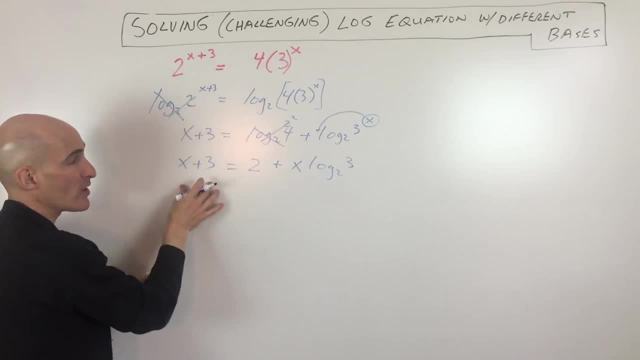 Okay, so we're getting closer. we want to group the x terms on one side, we want to get everything else on the other side. So what we're going to do is we're going to subtract this x log base 2 of 3, so that's going to be x minus x. log base 2 of 3 equals 2, and I'm going to move the 3 over here by. 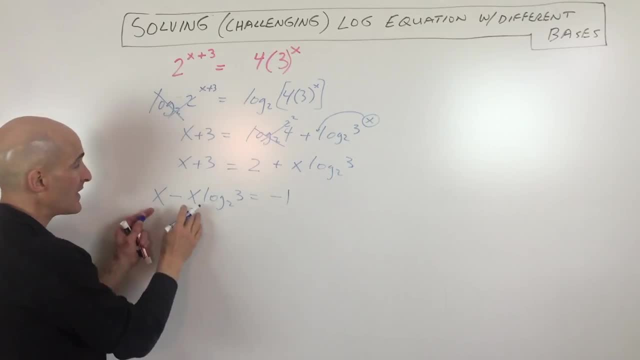 subtracting 3 from both sides, that's negative 1.. Okay now what we're going to do? because we want to get the x by itself, we're going to factor it out of both of these terms. So we're going to factor out the x, which leaves us with 1 minus log base 2. 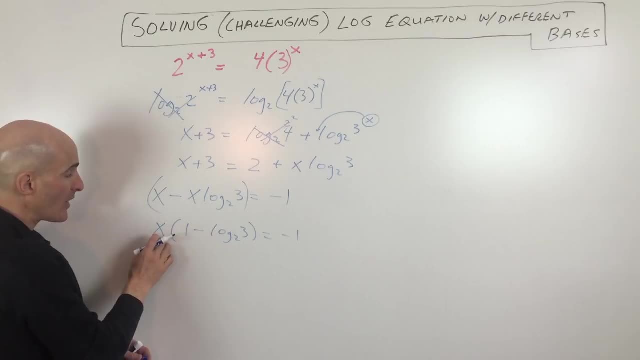 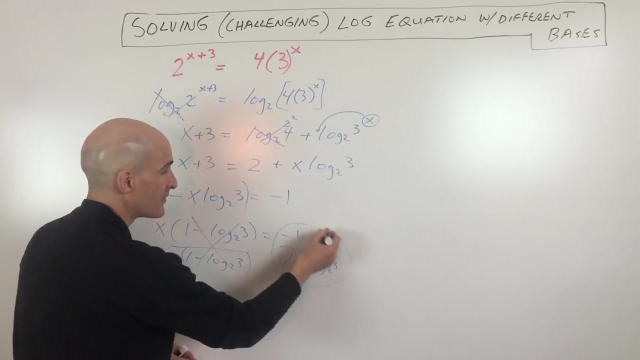 of 3. okay, equals negative 1, and now all we have to do is divide by this proportion here that we don't need. okay, and don't want. both sides. keep it balanced: 1 minus log base 2 of 3.. These are going to cancel and you can see, x equals this quantity here. So this is a calculator ready answer. 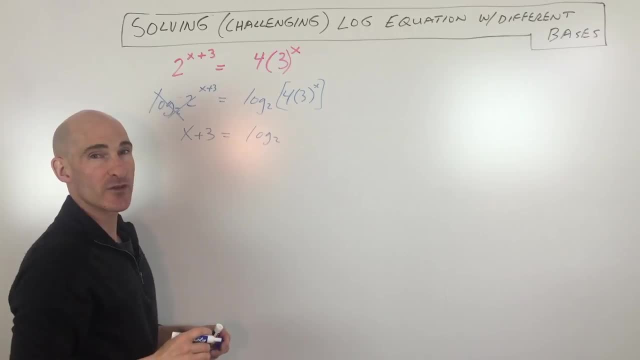 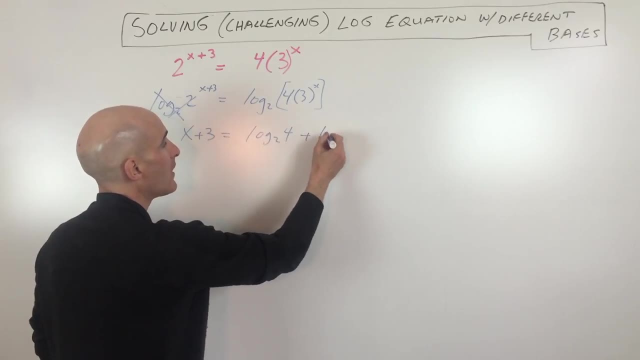 what we're going to do now is because these are multiplied together, the 4 and the 3 to the x. we're going to use the properties of logs to expand this. So this is going to be log base 2 of 4 plus log base 2 of 3 to the x power. Okay, now we're going to continue on. We're going to take 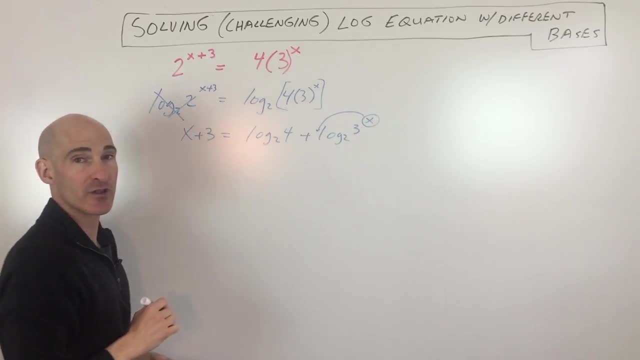 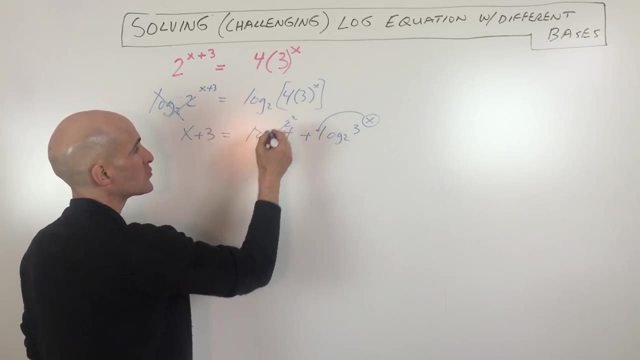 this exponent: use the power rule for logs. You're going to bring that down in front of the log. Okay, 4 is really like 2 squared. Okay, so log base 2 and exponential base 2- those cancel, Those are inverses. so we're left with 2.. Over here we have x log, base 2 of 3. Okay, and x plus 3.. 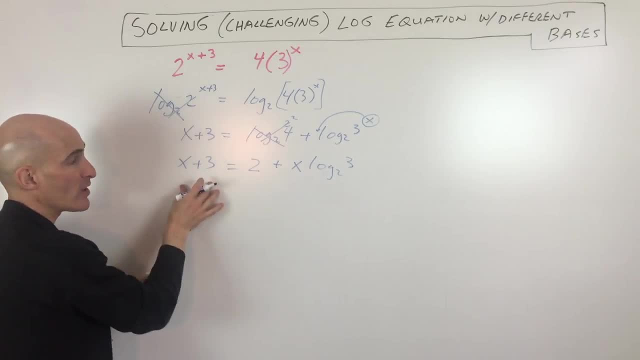 Okay, so we're getting closer. We want to group the x terms on one side, We want to get everything else on the other side. So what we're going to do is we're going to subtract this x log, base 2 of 3.. 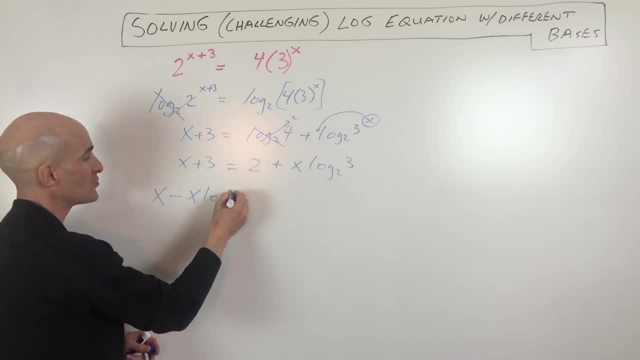 So that's going to be x minus x. log base 2 of 3 equals 2, and I'm going to move the 3 over here by subtracting 3 from both sides. That's negative 1.. Okay, now what we're going to do? because we want to get the x by itself, we're going to factor it out. 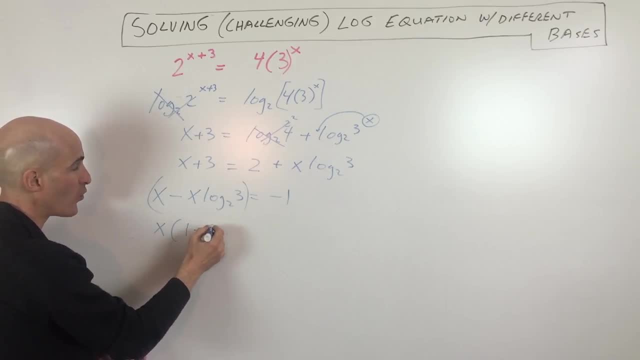 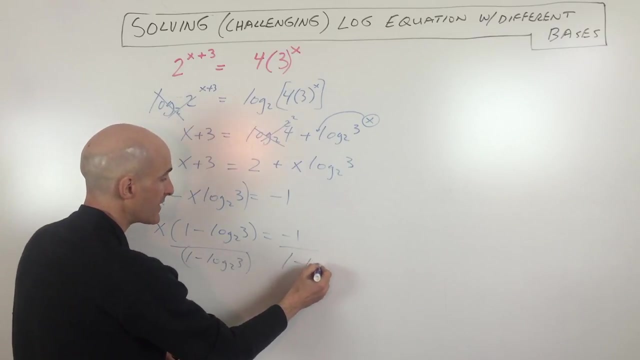 of both of these terms. So we're going to factor out the x, which leaves us with 1 minus log base 2 of 3.. Okay, equals negative 1, and now all we have to do is divide by this proportion here that we don't need, Okay, and don't want Both sides keep it balanced: 1 minus log base 2 of 3.. These are: 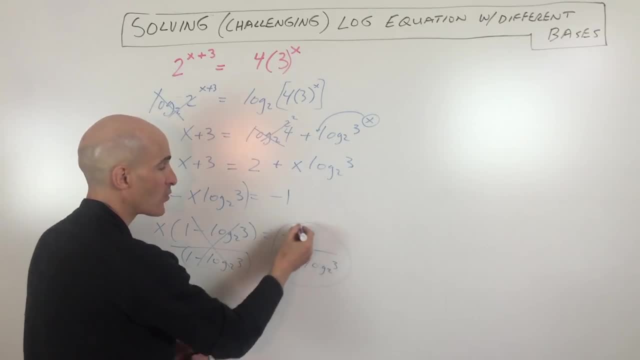 going to cancel and you can see: x equals this quantity here. So this is a calculator ready answer. You can go ahead and put it in your calculator to get a decimal approximation, but this is exact. So I hope this example problem gave you a better understanding about how to work with logs. 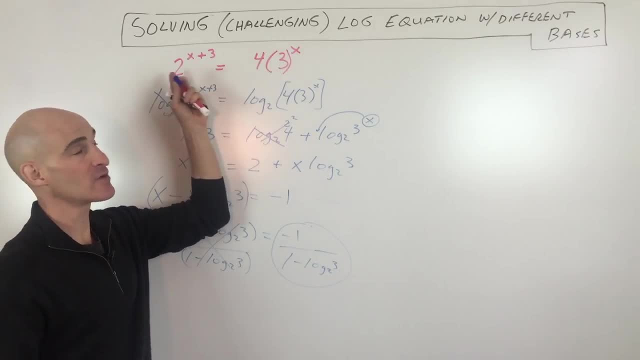 especially when you have different bases- Okay, like we had base 3 and base 2.. If you're enjoying these videos, subscribe to the channel. Go ahead and check out some of my past videos on logs and some of my other videos as well, and I look forward to seeing you in the next video. I'll talk to you soon.